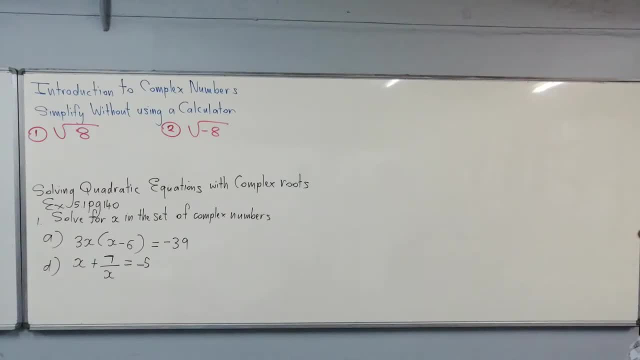 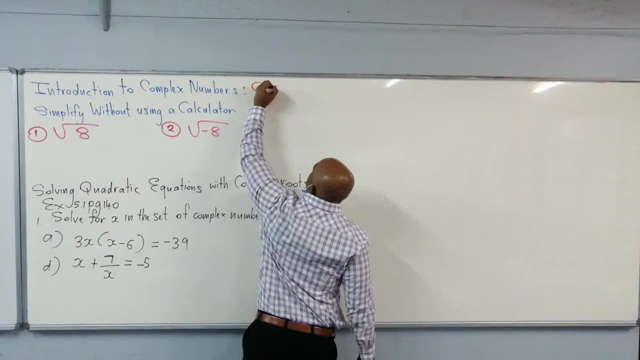 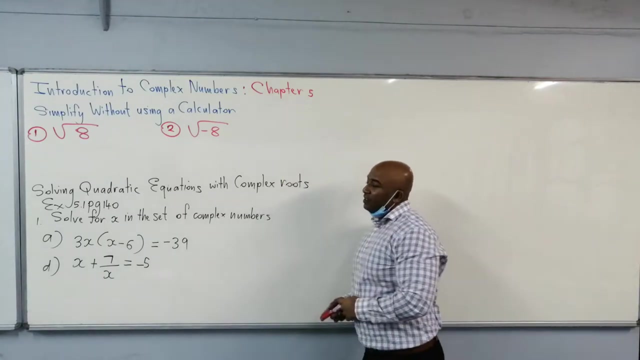 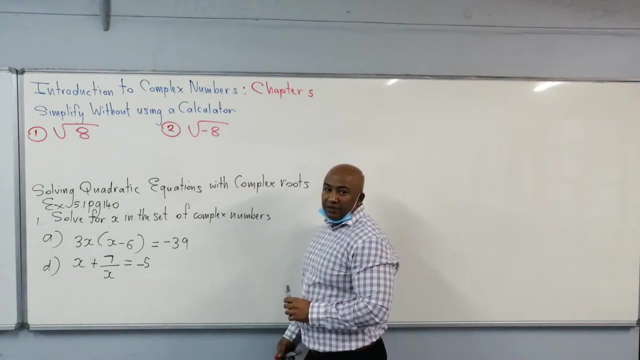 Okay, so now we are dealing with complex numbers, so this will be chapter 5 in your textbook. So we are dealing with complex numbers. We're moving straight to complex numbers because electrical students- they need to be using some of the rules that we're going to learn. 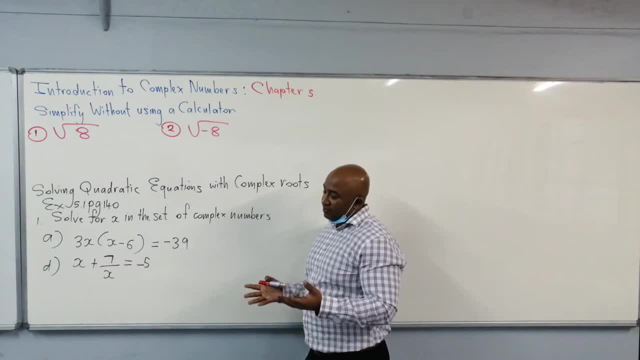 here in the industrial electronics that subject- and electrotechnics dealing with alternating currents. So there's a lot of applications for this Right. but let's have a look at you. haven't dealt with complex numbers before, so let's. 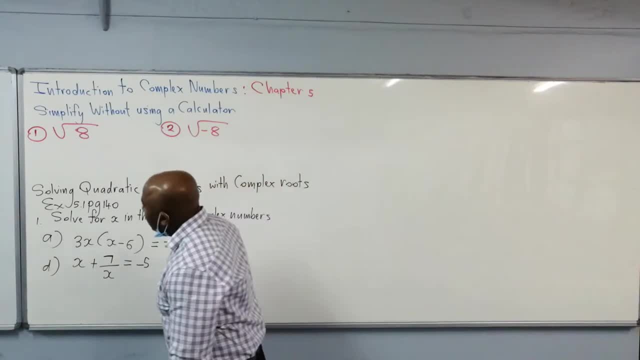 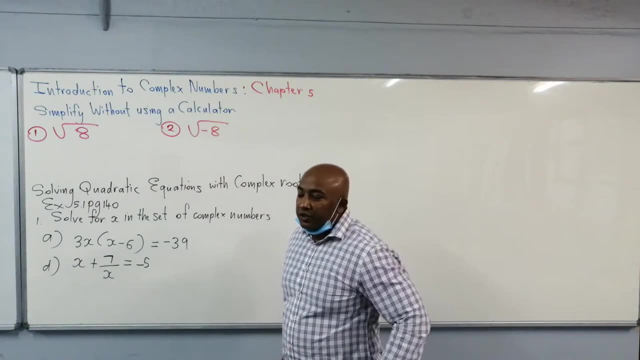 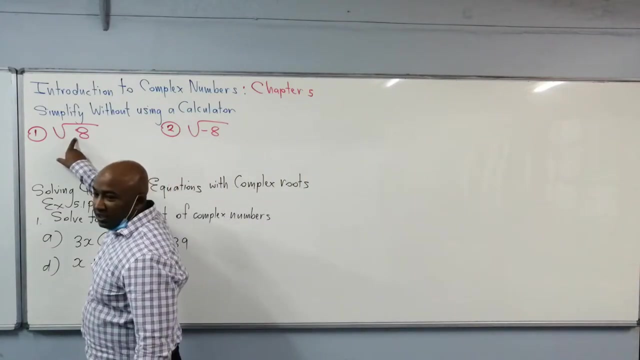 have a look at these two examples here from M3.. If I asked you to simplify the square root of 8 without using a calculator, Then the fact that you see square root here, that means we need to have a perfect square. Okay, like the square root of 4, that's a perfect square, which is 2.. The square root: 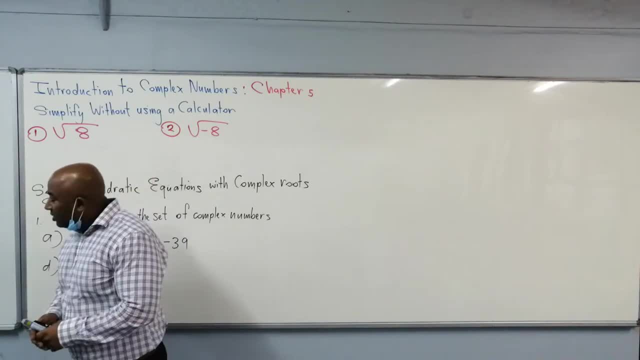 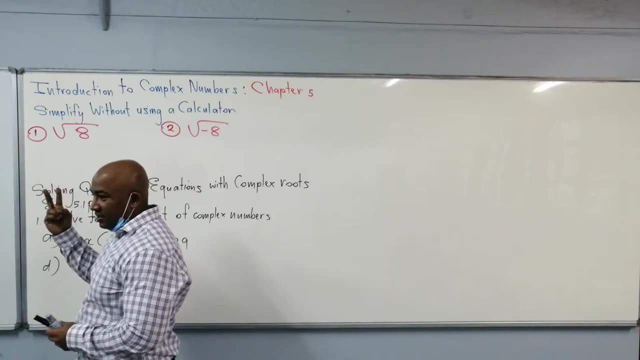 of 25 is 5.. The square root of 100 is 10.. So what do we do? We rewrite 8 as two factors. Okay, one of those factors then has to be a perfect square. So, from our time table, 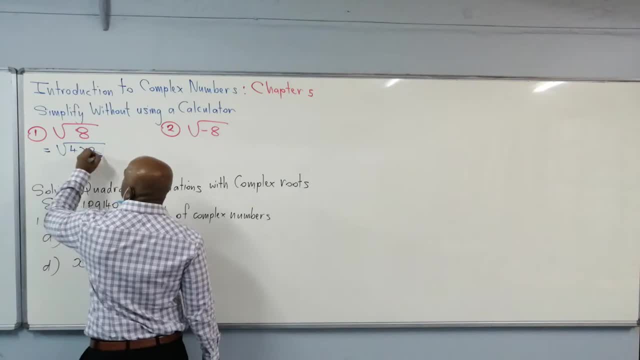 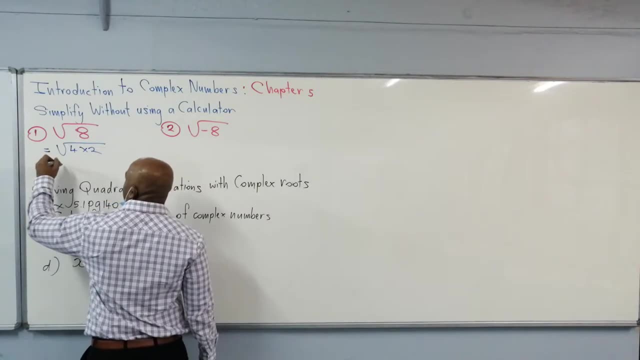 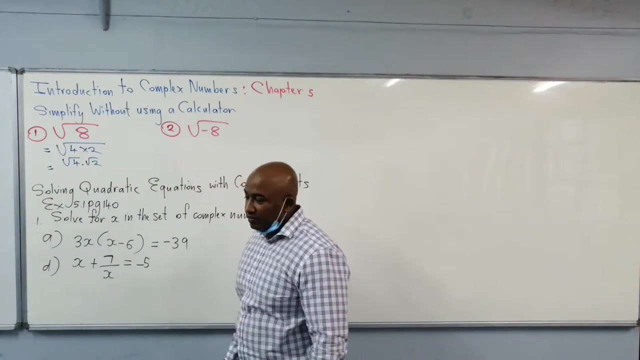 Okay, we know that 8 is the same as 4 times 2.. Right, so now from our exponent laws, then we know that this can be written as the square root of 4 times the square root of 2.. And we know the value of the square root of 4. 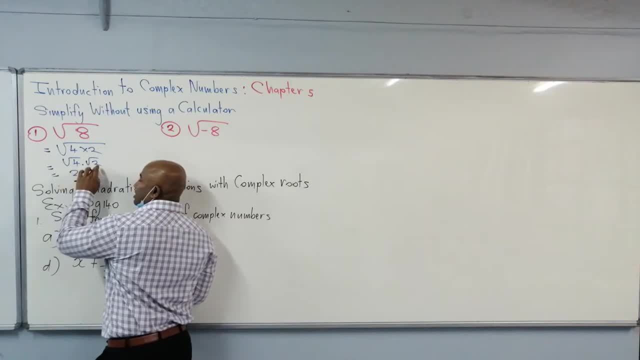 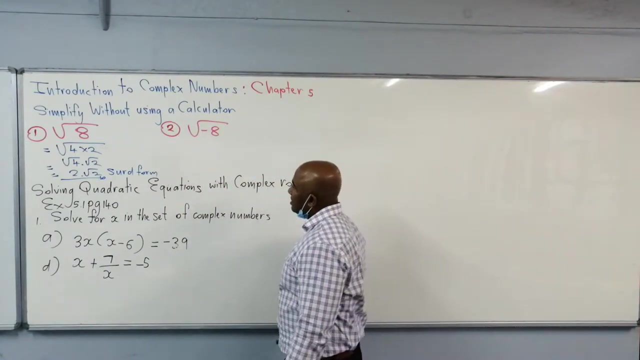 without using a calculator is 2, and this we do not know. so we multiply it and we leave it in set form. So that is 2 root of 2.. Okay, we've been dealing with that from school. Now, in school when you had a square root of a negative. okay, so previously we would. 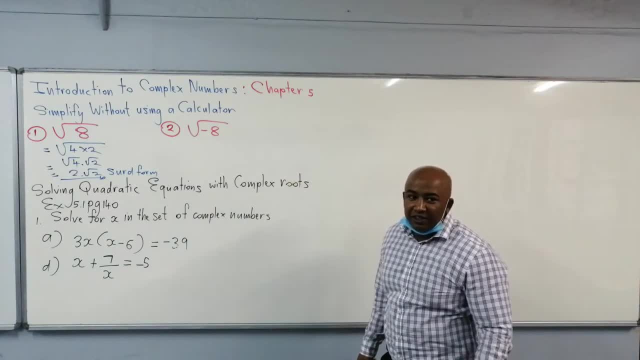 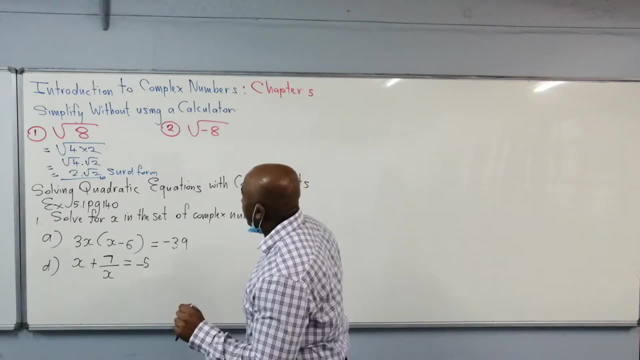 just say it's undefined. Okay, now it's no more going to be undefined. We are now going to be using a substitution for the square root of 2. For the square root of a negative. So what am I saying? We use a substitution. 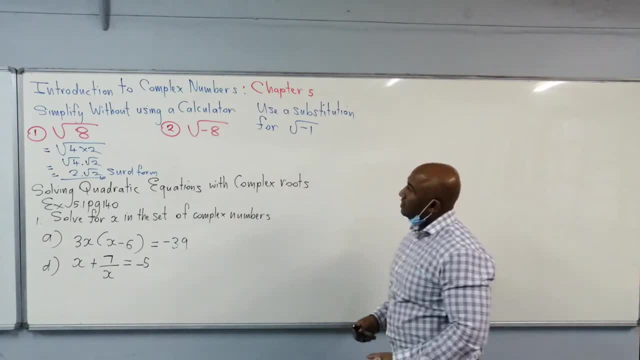 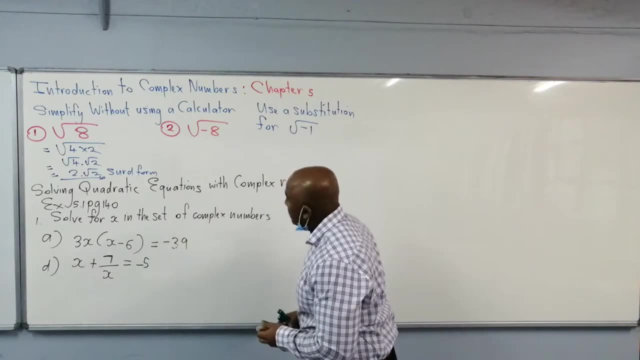 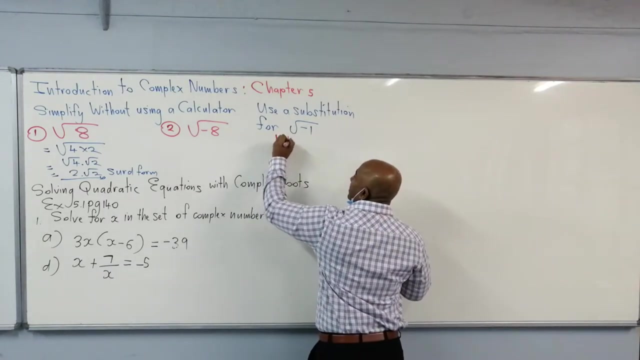 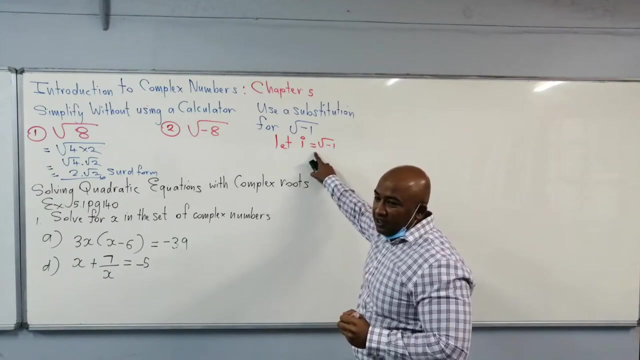 For the square root of minus 1.. Okay, So the letter that we use, or most of the textbook uses, is the letter i or j, So I can say x, i, equal to the square root of minus 1. but now because of, look in the text in the maths textbook. 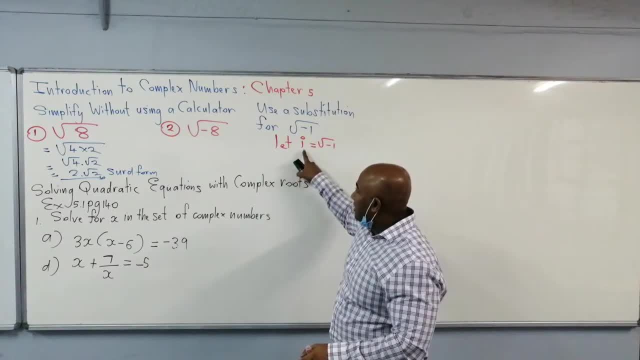 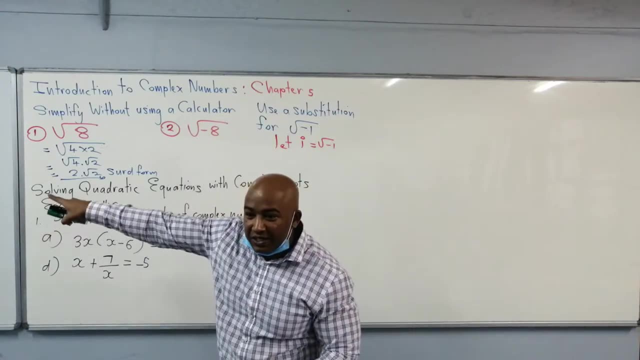 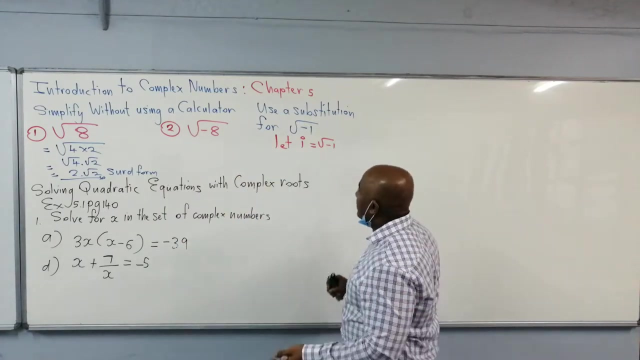 they use both i sometimes, j sometimes. but the reason why we prefer not to use i? because it confuses the electrical students, like you know, when you're finding out i1, i2, i3, the current i also stands for current in engineering science, and all that so you can use the symbol. 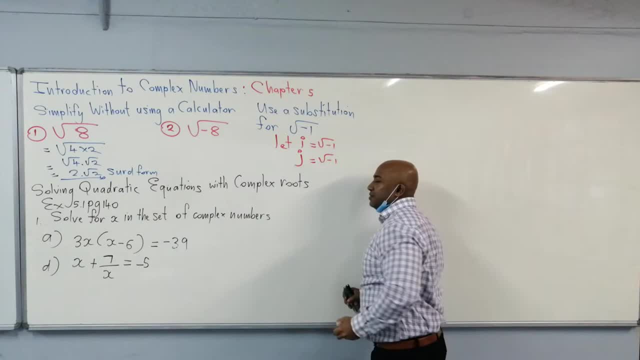 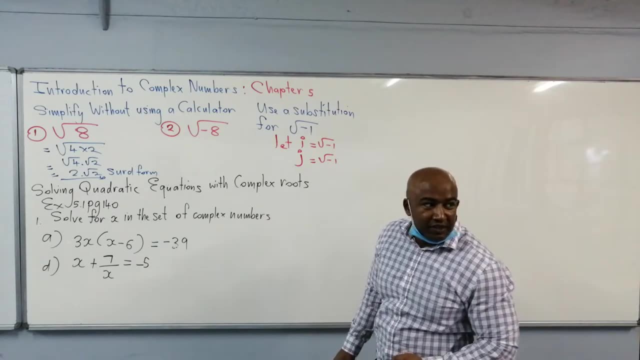 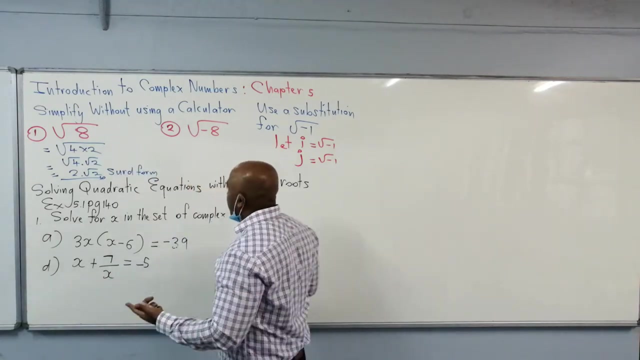 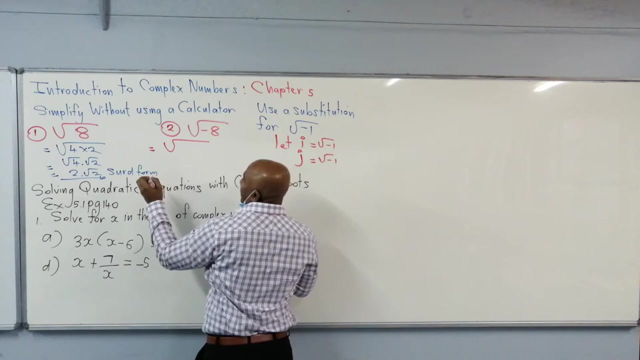 j, you'll find j equal to the square root of minus 1. okay, so now how do we use it in a situation like this here? so we got the square root of minus 8. we follow the same simplification program. so what's happening here now is you- this is equal to you- got the square root of 8. 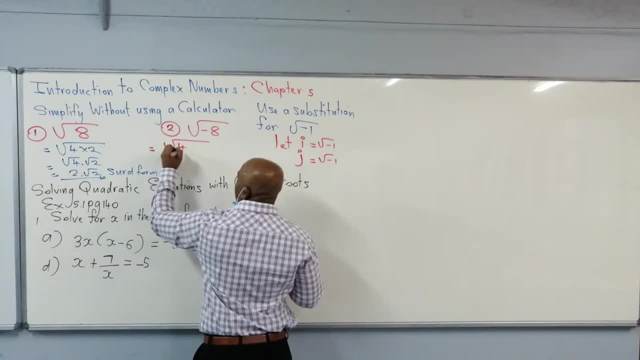 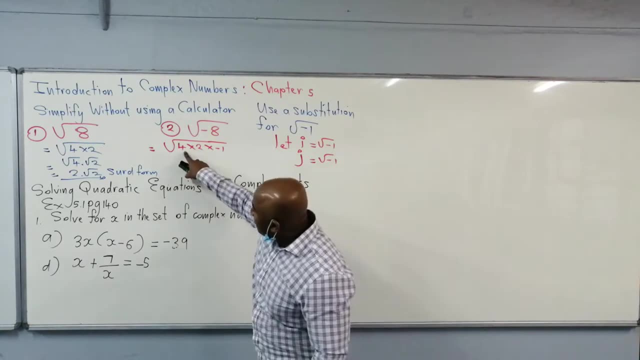 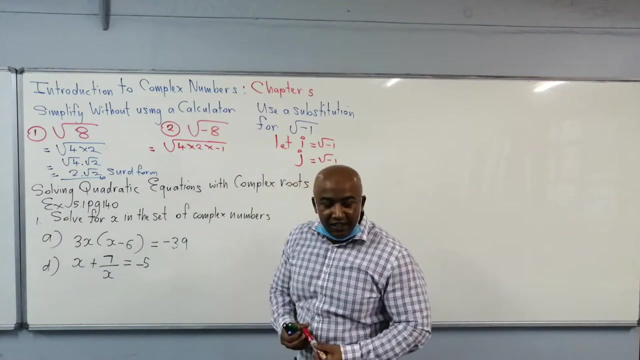 so that's going to be 4 times 2 times minus 1, because 4 times 2 is 8 and 8 times minus 1 will give you minus 8. it's still a negative 8. right now. what will happen is this can be broken up into square root of 4. 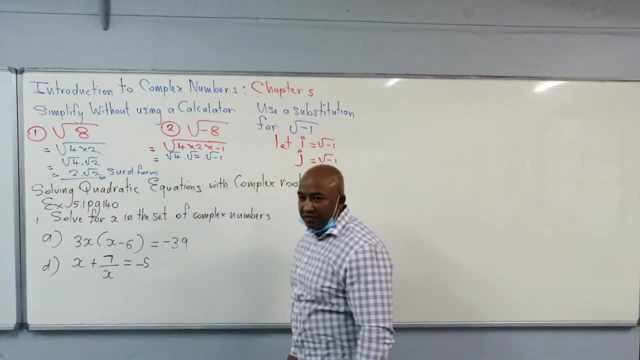 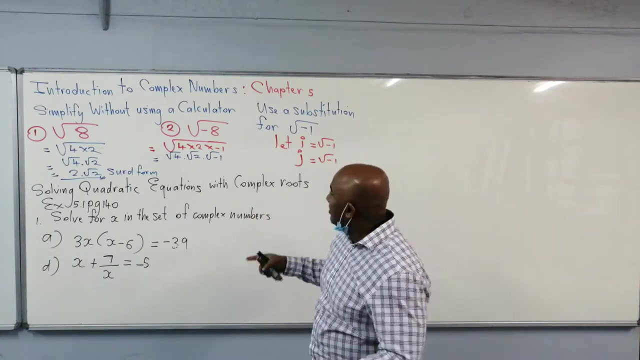 times square root: 2 times square root: negative 1. so what do we know? now, on the side of your page you're going to let i, if you want to, or j, both are correct. you will not be penalized, okay, but it's sometimes it's better to use j than high. also why? because sometimes you might. 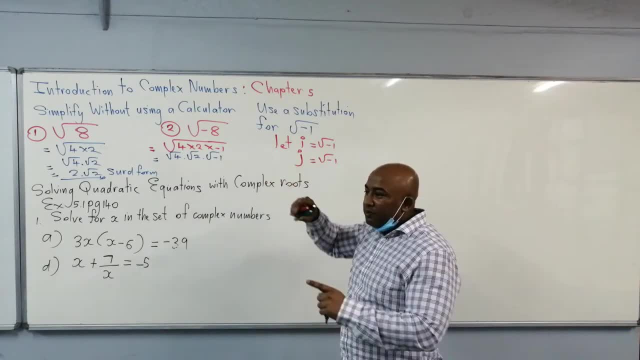 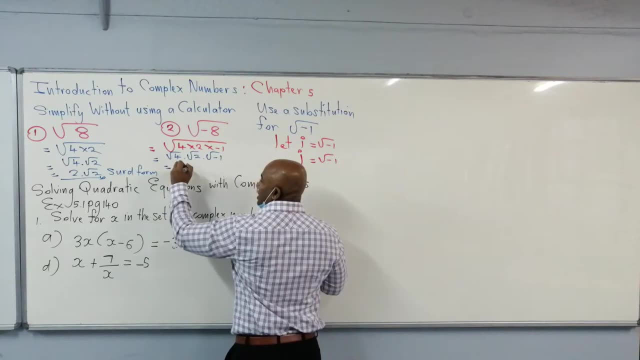 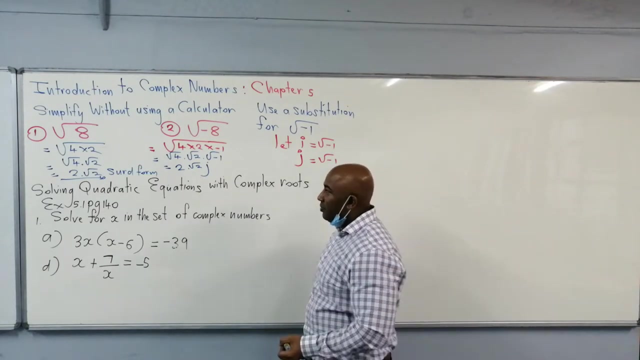 think there's a high. when you look back it's a one. you might mistake a one for a high depends on how you're writing. so this is the square root of four, which is two times root, two times. i'm gonna write down j? okay. so every time we see the square root of negative one, we are going to be substituting. 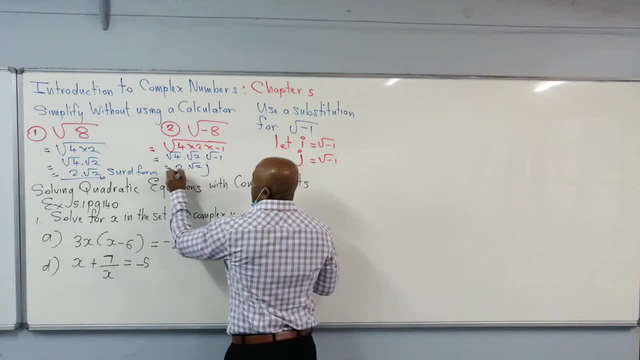 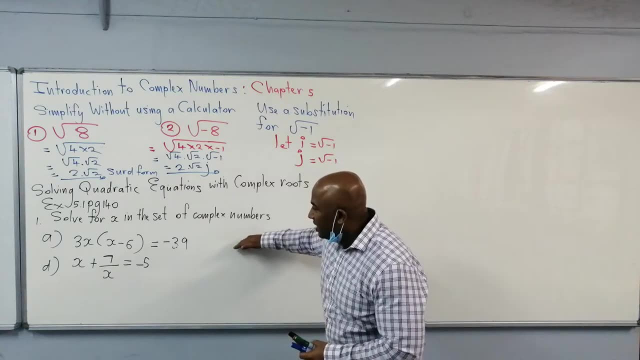 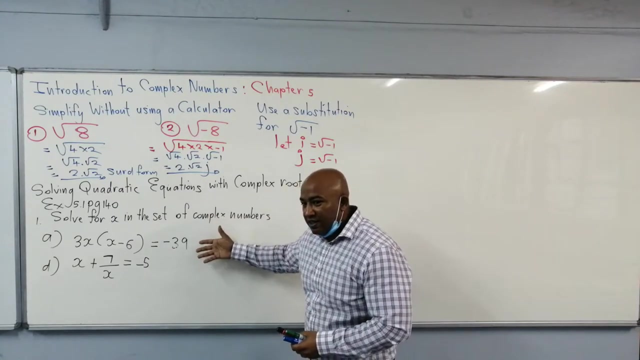 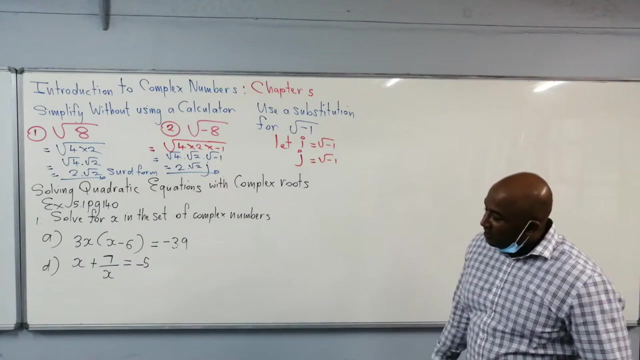 j or i. all right, so that is for now. it's a new concept to you, so copy this down. and now let's see how we're going to work out quadratic equations that we have done previously- solving for x- without using a calculator. okay, so copy this down. write down the first one here. 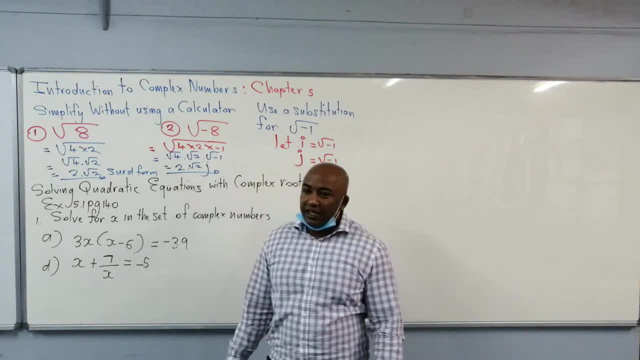 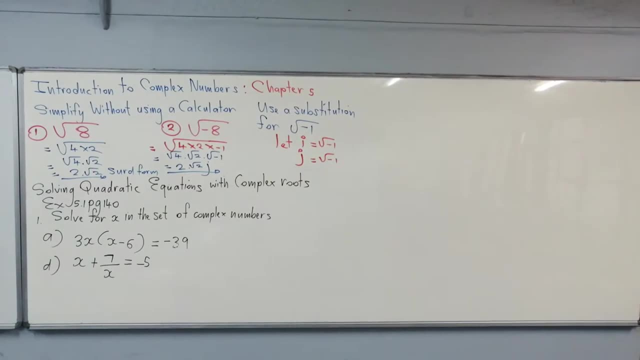 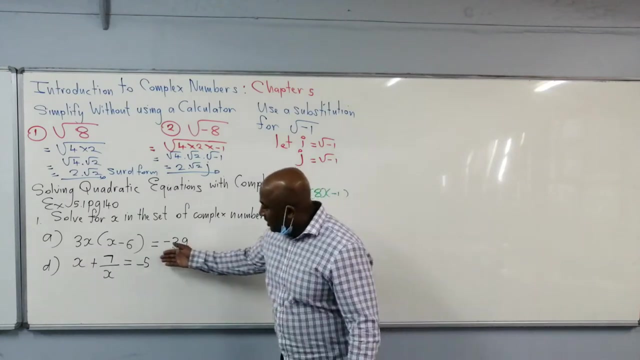 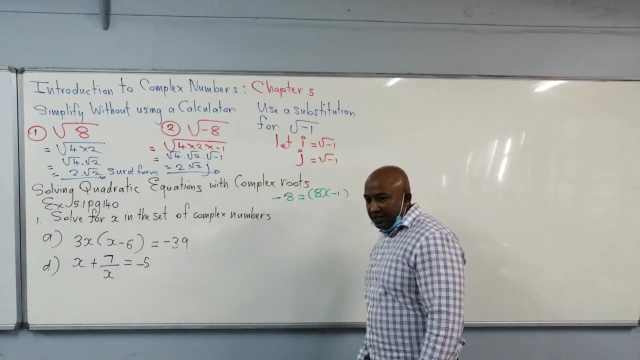 solve for x. let's see what you can do: solve for x without using a calculator. so in this exercise we have into these two equations: solve for x. so what do we do? you won't be told in the exam that this is an equation that involves complex numbers. you need to rearrange the equation. you need to try and work it out. 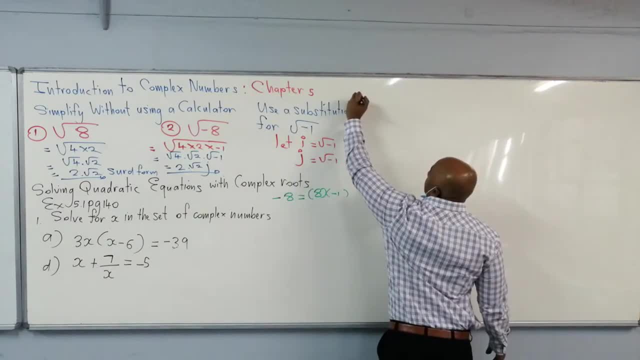 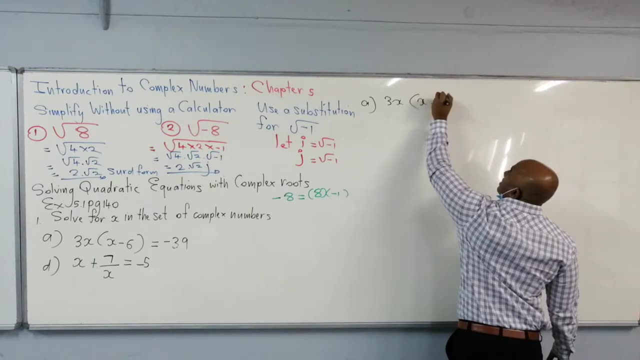 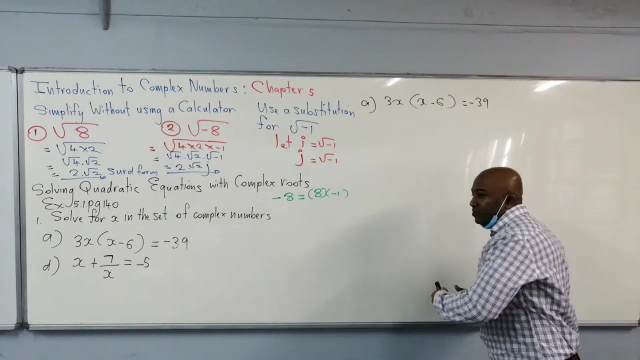 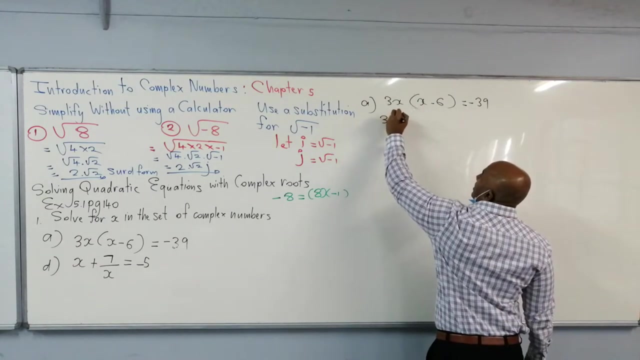 so let's take the first one. so we have 3 x and then you have x minus. multiplied by x minus 6 is equal to minus 39. so what do you normally do? you normally remove the brackets and rewrite your equation in standard form: 3x times x will be 3x squared, 3x times minus 6 is minus. 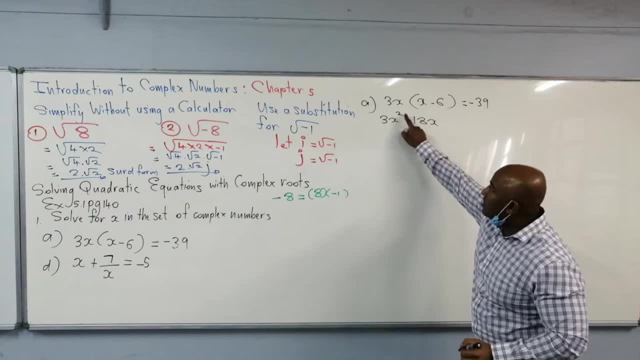 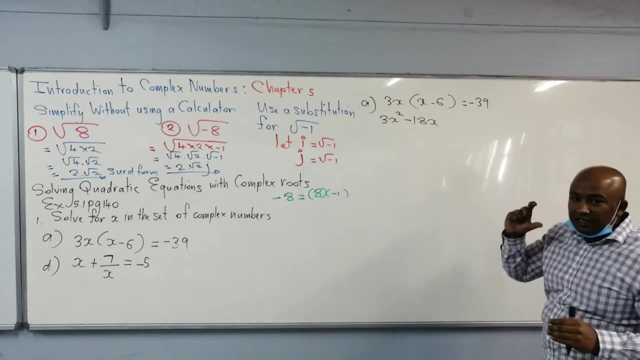 it's in x, and then your constant. here you have a square and the second variable has a power 1, this is a quadratic. so always make your quadratic equal to 0. so that's plus 39 equals to 0. and what do you do now? you try and make it. 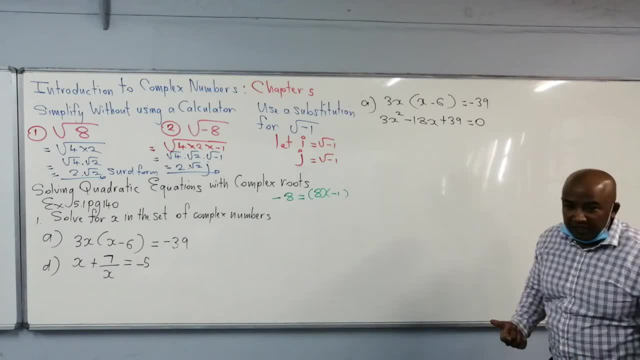 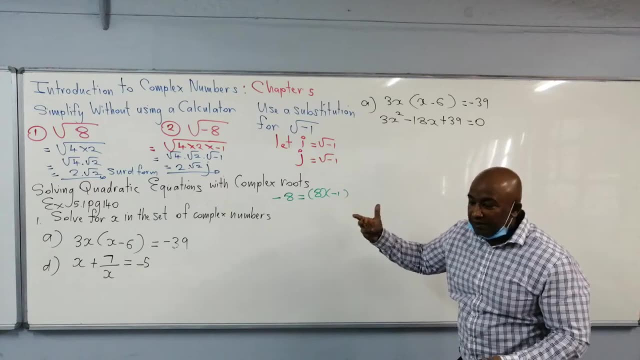 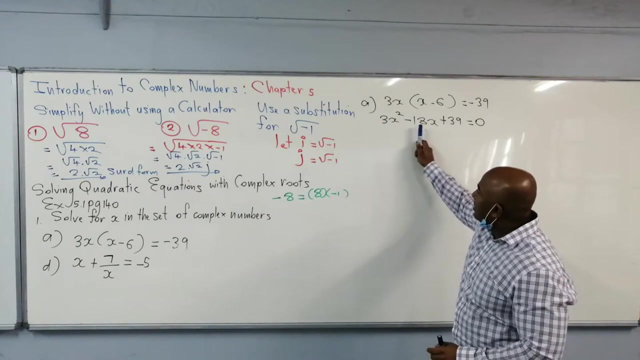 simpler to factorize. you don't have to do that, ok, but you can. can we divide by 3? is it possible? you don't have to do that, but is it possible, yes or no? let's check. 3 can go into 3 one time. 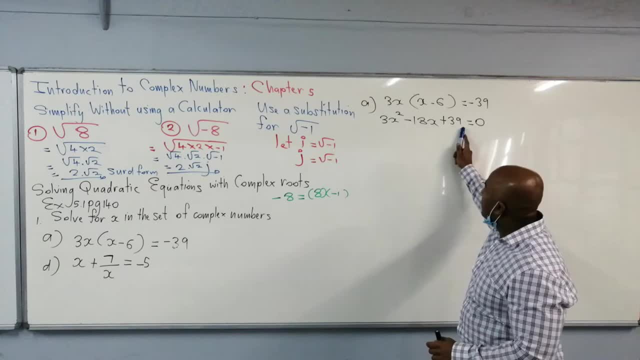 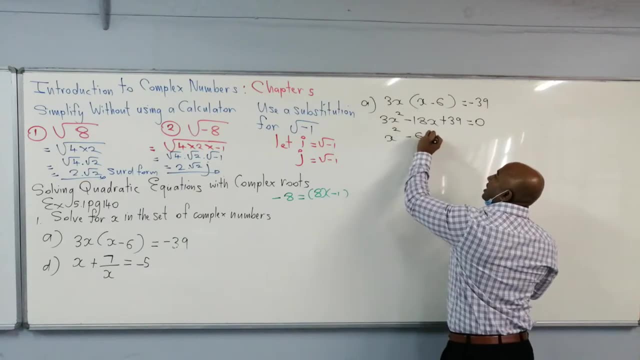 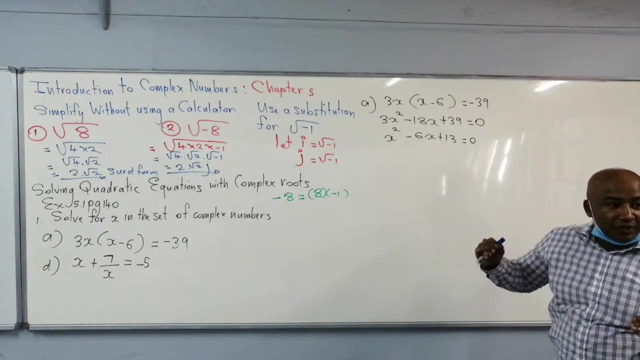 can 3 go into 18. 6 times can 3 go into 39. so it is possible. so let's just divide today. so therefore it's going to be x squared minus 6x plus 13 equals to 0, not compulsory, but normally this is what we do. 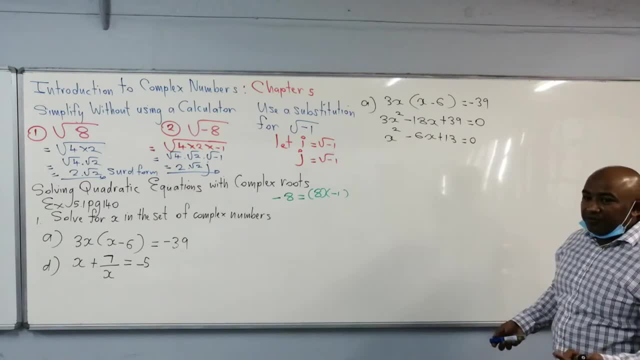 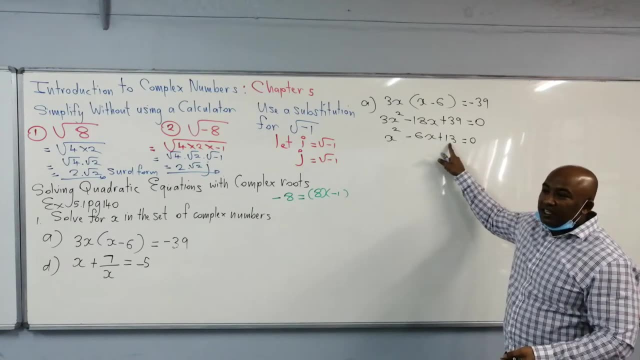 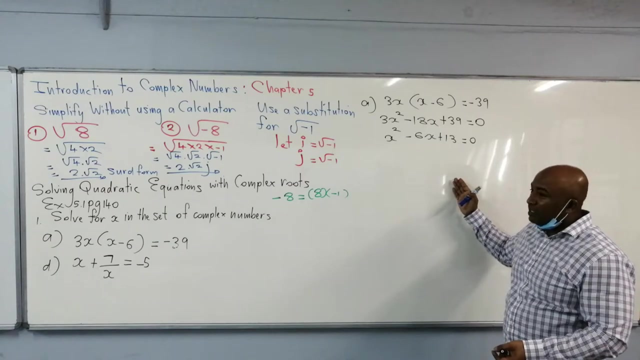 we always try and make it simpler. we try and factorize. now is it possible to factorize it? what are the factors of 13? 13 is a prime number. it's only 13 and 1, only 13 and 1- a prime number. remember, it has only 2 factors. 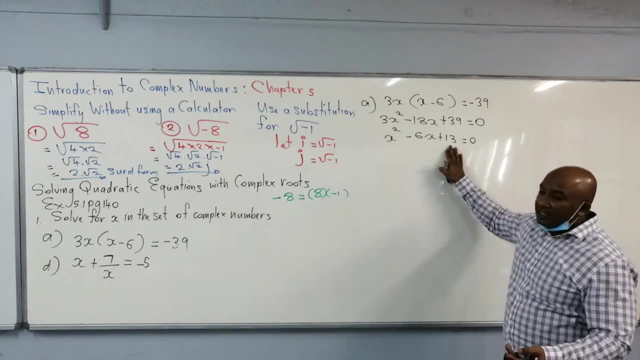 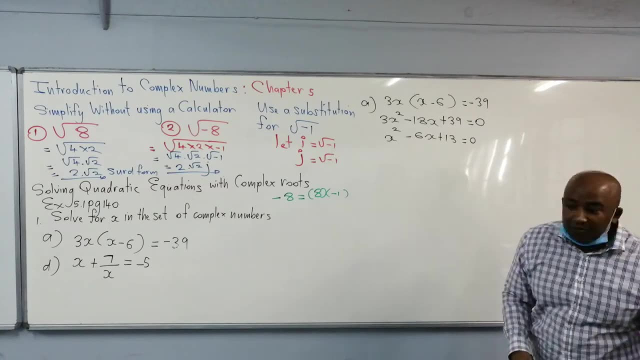 the number itself and 1. this cannot be factored. 13 is 13 times 1. will I ever get a negative 6? no, that means this cannot be factored. so it cannot be factored. so it cannot be factored, so it cannot be factored. 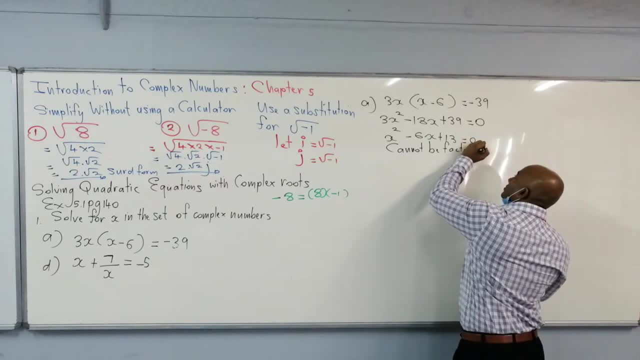 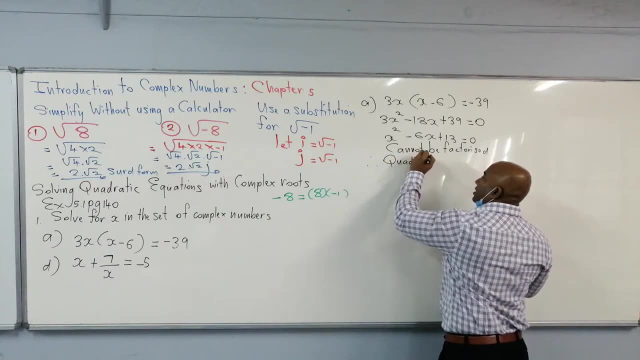 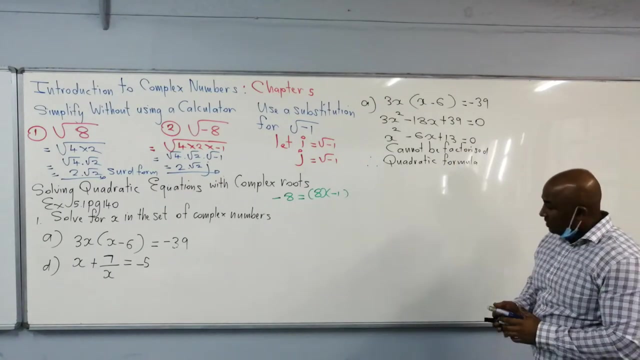 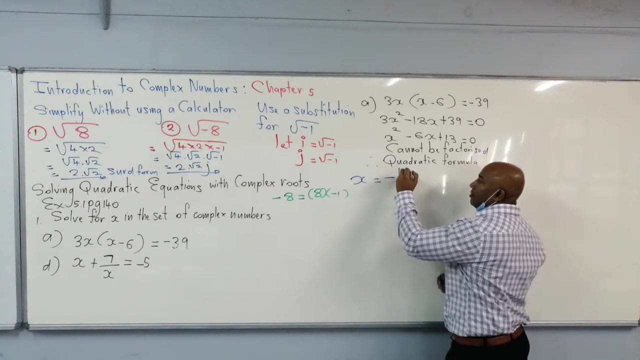 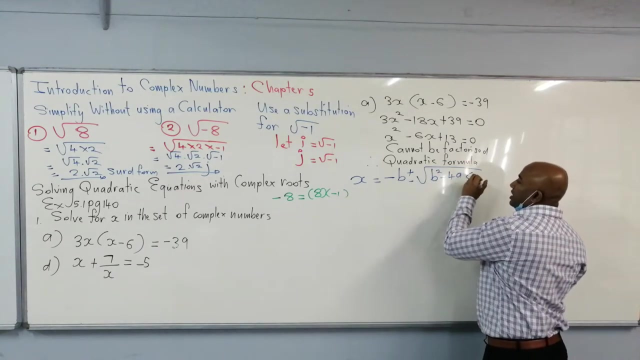 so, therefore, I need to use the quadratic formula. I will have to use the quadratic formula. so what is the quadratic formula? x is equal to minus b, plus or minus. the square root of x is equal to b squared minus 4ac all divided by 2a. 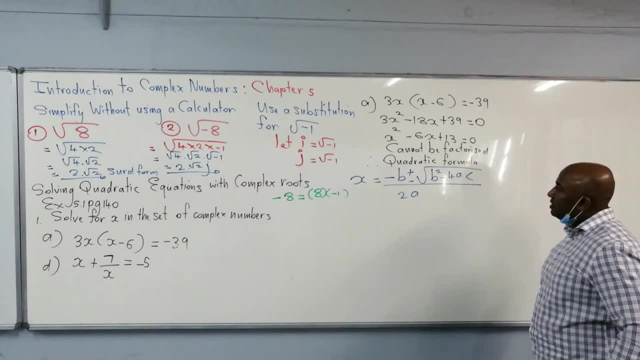 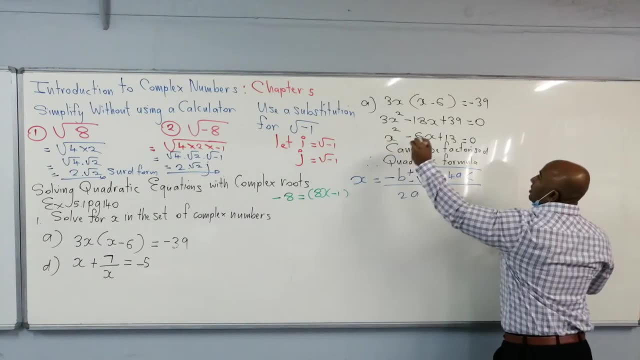 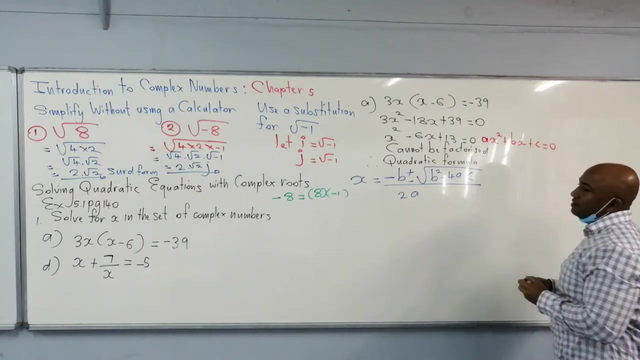 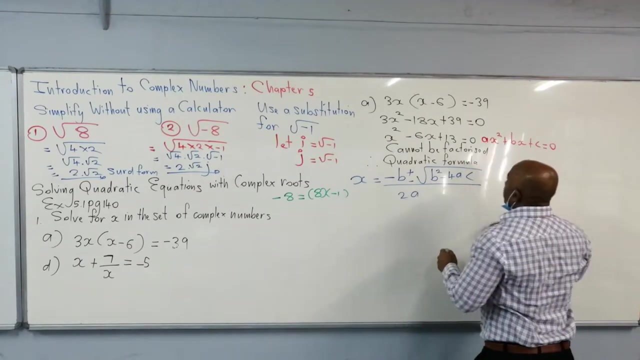 so identify your a, b and c. so remember: a is the coefficient of x squared. so remember we have ax squared plus bx plus c equals to 0. so a is the number that's multiplied by x squared, which is 1. b is the number that's multiplied by x. 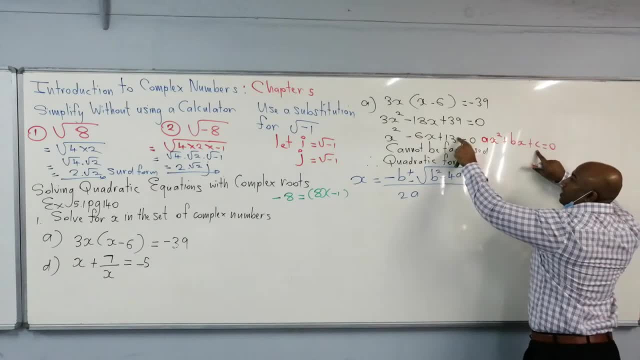 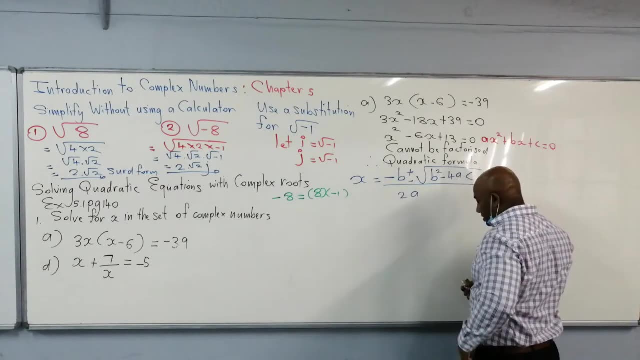 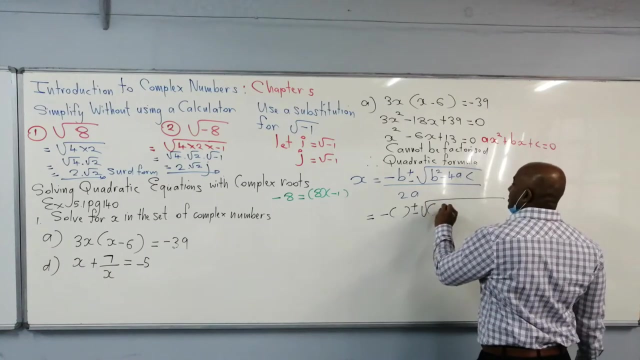 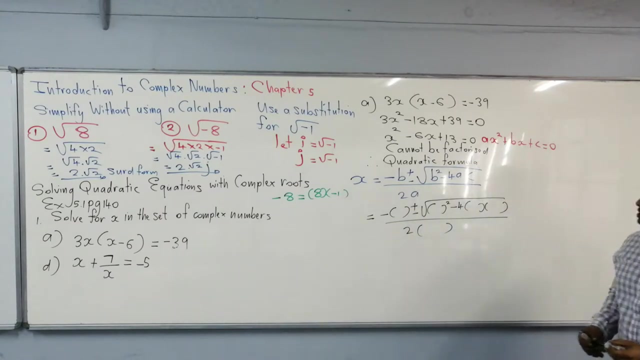 the coefficient, which is negative, 6, and c has no x, it's just a number, a constant 13. so now let's substitute minus b, plus or minus the square root of b, squared minus 4 times a, times c, all over to a. so what is my b now? 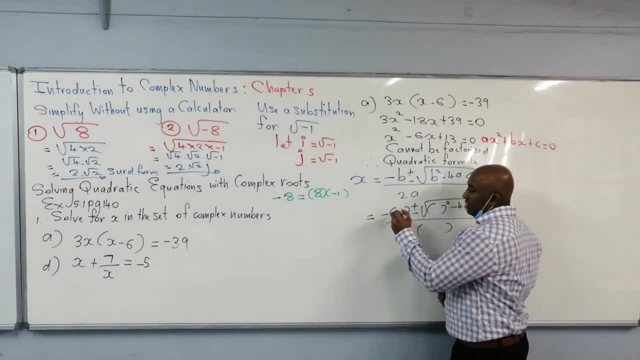 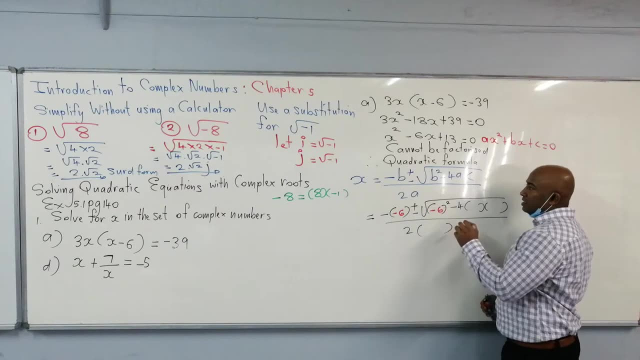 b is minus 6. then we have b again, which is minus 6, a is 1 and c is 13. right, all divided by 2 times a, which is 1, substitute into the quadratic formula b, which is 1, and c is 13. 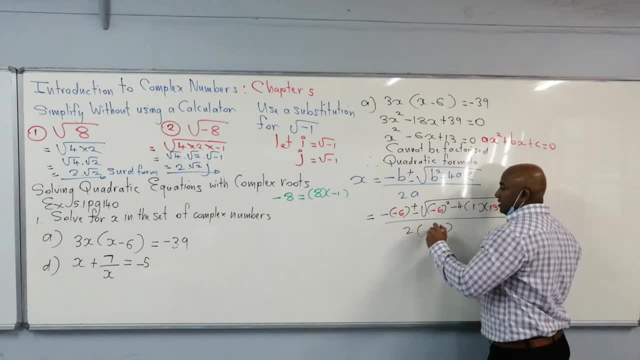 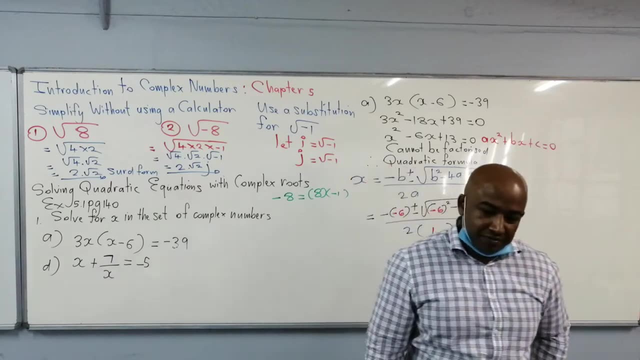 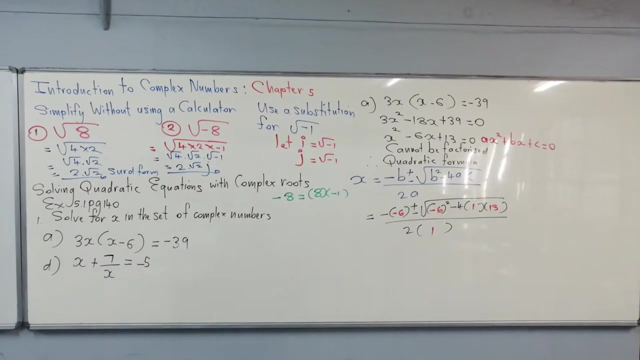 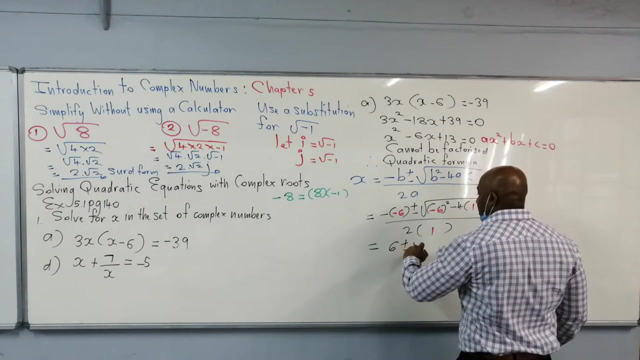 right. all divided by 2 times a, which is 1, substitute into the quadratic formula a, which is 0. let's see what we get right. so let's see what we get. we get a negative times a negative, which is positive, 6 plus or minus. the square root of negative, 6 squared, is: 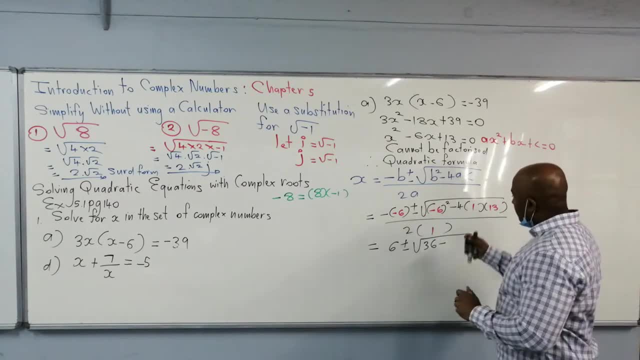 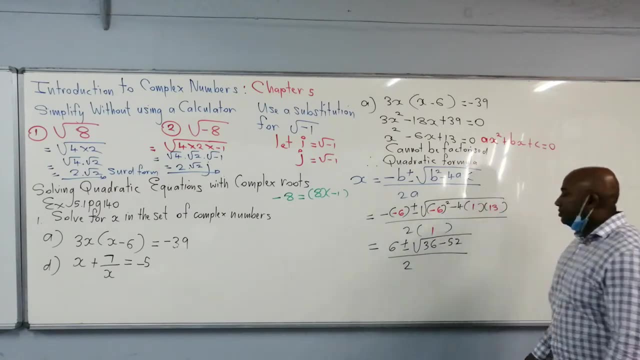 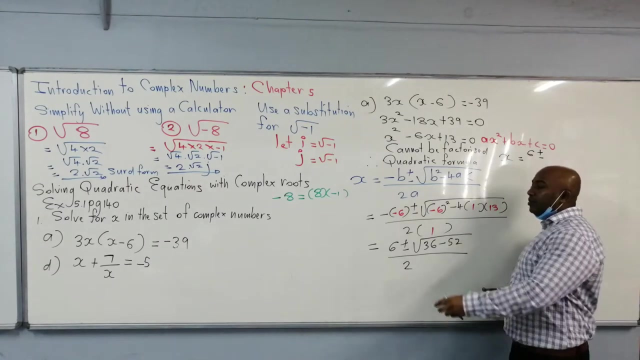 36 minus. what is this here? all divided by 2, so now? so X is equal to 6 plus or minus. so, on the calculator, remember to not go and do the whole thing, you're gonna get an error. you will just type out this part, that part, and you type this whole thing out, and then you will get your answer. 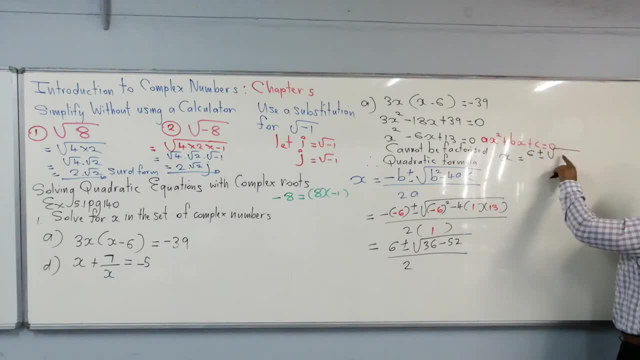 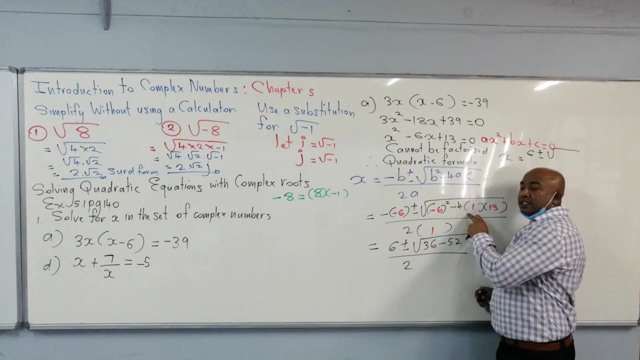 so, therefore, we get 6 plus or minus the square root of what. what do you get here? what do you get? you mean the calculator doesn't get it. well, get out. I just said, type this out inside the square root. it means you must not include the square root in your calculation. 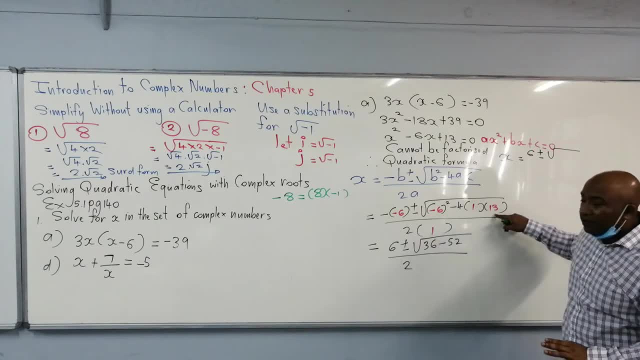 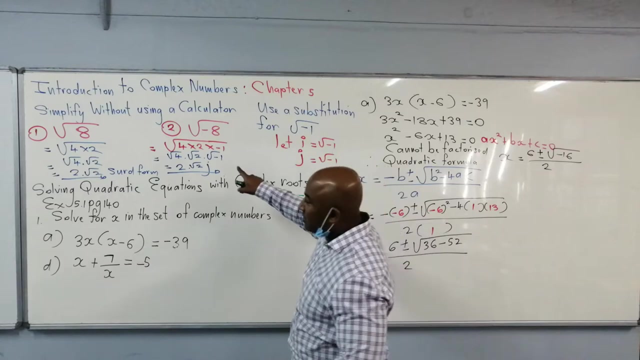 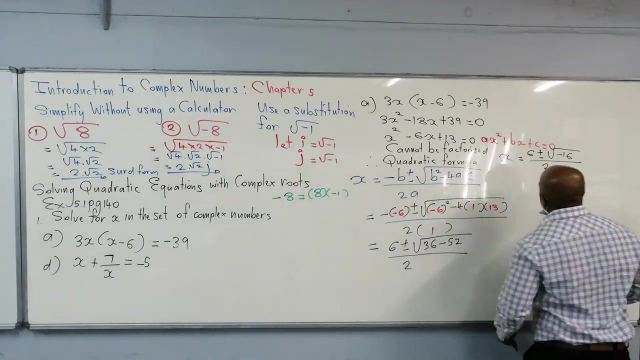 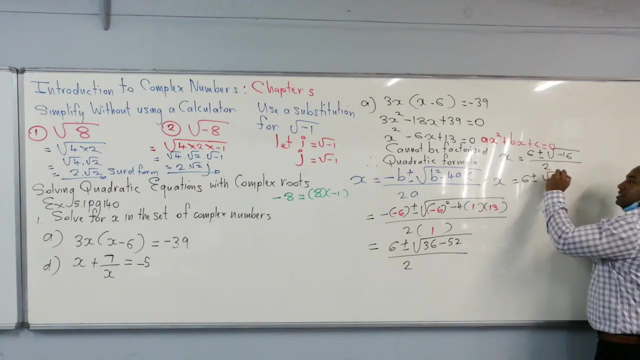 forget about this. forget about that. just type this part out. only what do you get? minus 16 all divided by 2. now, now remember what we did here when we had minus 8. we need to do the same thing here. we got minus 16, so we're gonna go. X is equal to 6 plus or minus the square root of 16 times the square root of negative 1. 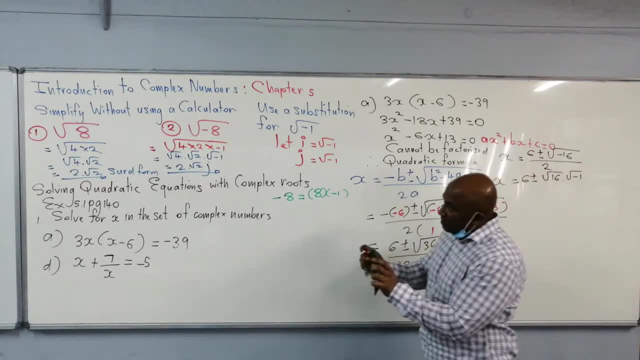 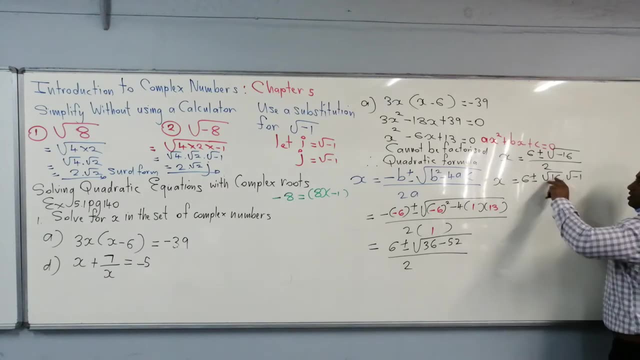 okay, we're dealing with S, w. if you have X, you can write it like this: if you have 8, it's gonna be 4 times 2 times minus 1. 16 is straight, perfect square, the square root of 16. so what am I doing? I'm going like this here. I'm going 16 times minus 1. 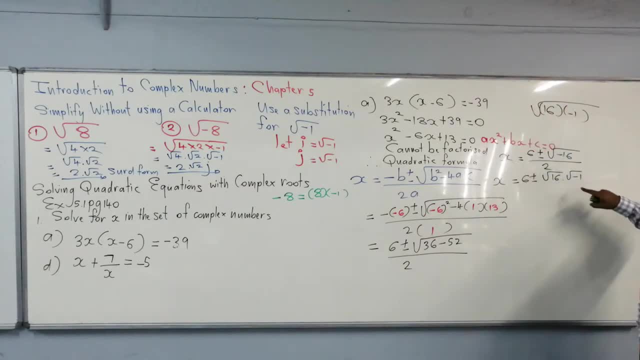 so therefore it becomes square root of 16 times the square root of negative 1 all divided by 2. now this is gonna be 6 plus or minus this. now you can use a calculator, but obviously it is a perfect square. you should know the square root of 16 is 4. 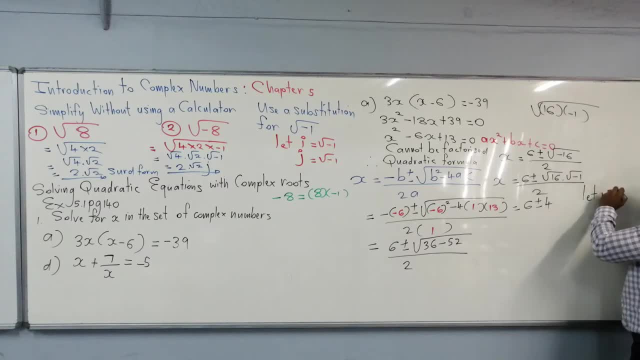 and then you will state: let the square root of minus 1 equal to j on the side of your page, there to show that you are using a substitution. this is now complex numbers, alright, so replace the square root of minus 1 with the symbol i or j. 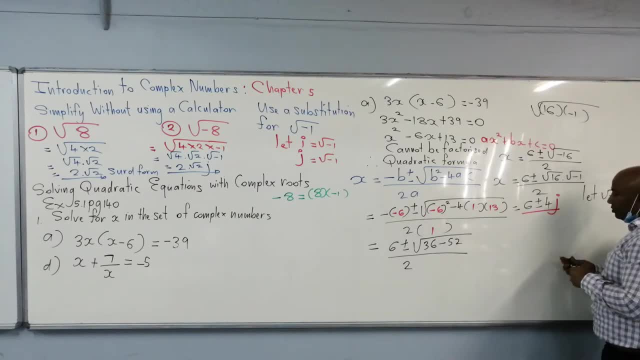 all divided by 2. now we need to simplify this fully for this question. ok, so I can separate this into 2 fractions. my LCD, my common denominator there is 2, so this can be written as 6 over 2, plus or minus 4j over 2. 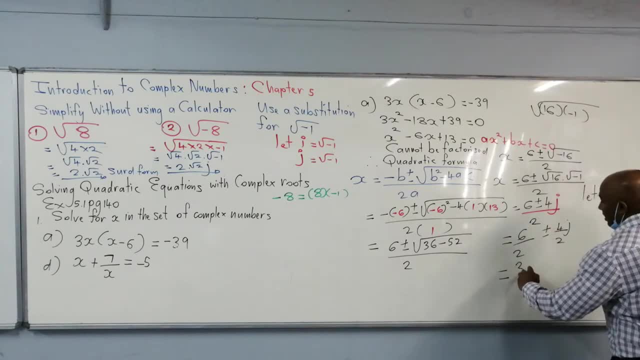 so 6 divided by 2 is 3, 4 divided by 2 is 2. so now this is simplified, so this is called rectangular form. I am going to explain this. I am going to explain the difference. there is 2 forms you are going to be dealing with. 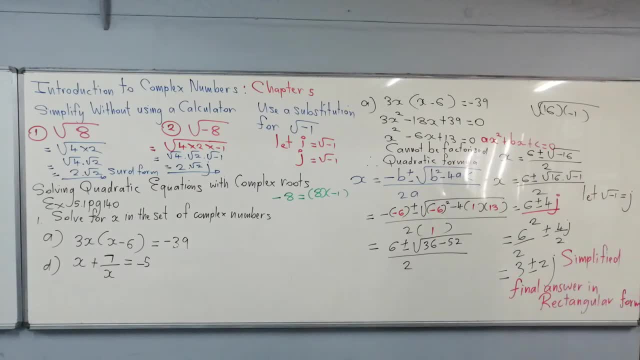 that is the next thing you are going to learn. so what happens here? you must simplify this fully. you don't leave it like this here. you must separate them completely. the number separated from the part with the j. can you see that you must have your real number here? 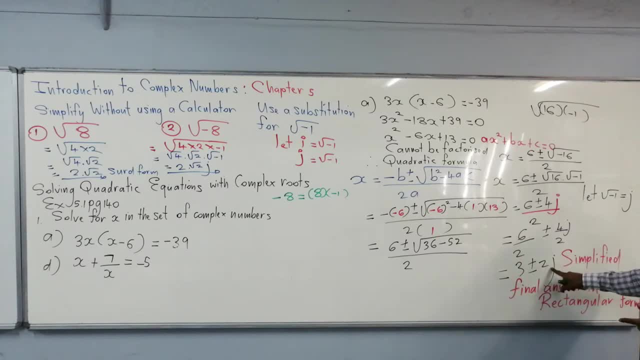 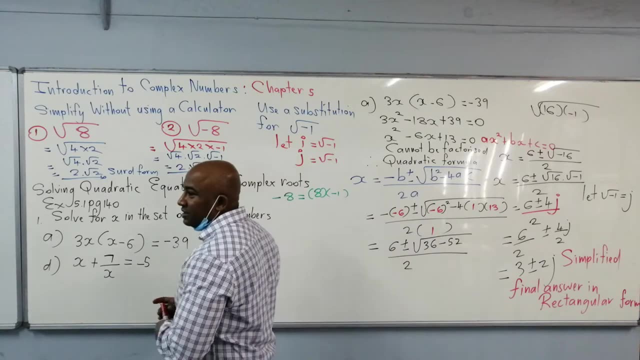 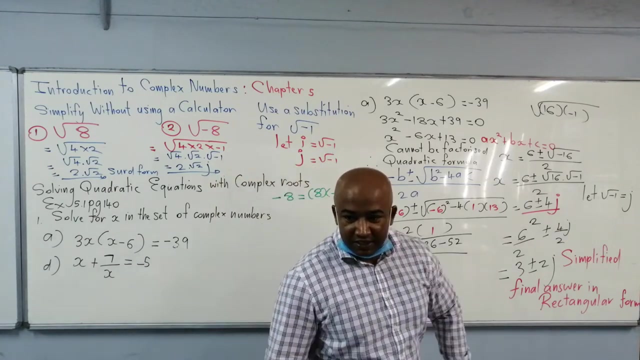 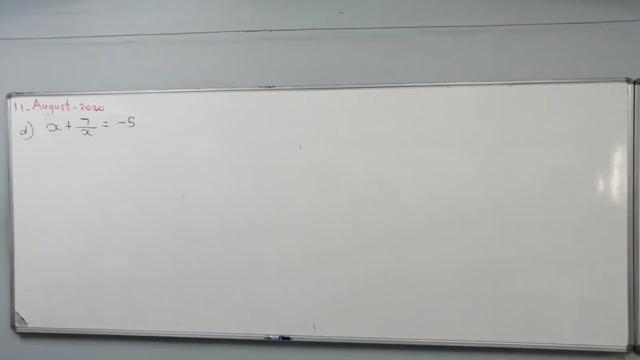 and the unreal part, or the imaginary part that is called the part with the j. how many minutes you got left here? ok, here is the next one. let's do this one d. alright, our next example. here we got x plus 7 over. x is equal to minus 5. 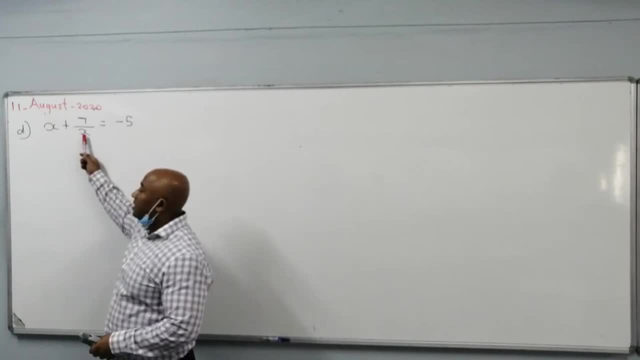 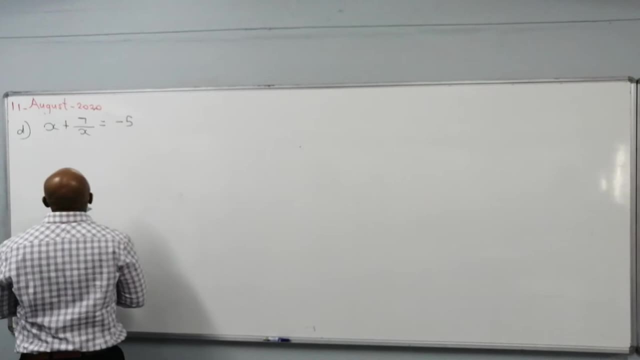 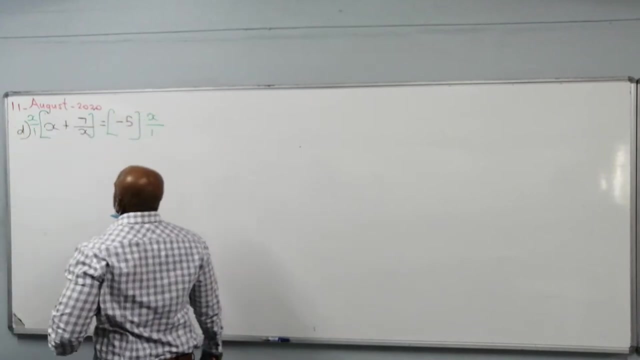 what can we do? we got x in the denominator, alright. so we don't want x in the denominator. so we can multiply. we can multiply by x over 1 on both sides. ok, you got x in the denominator. you know that x cannot equal to 0. 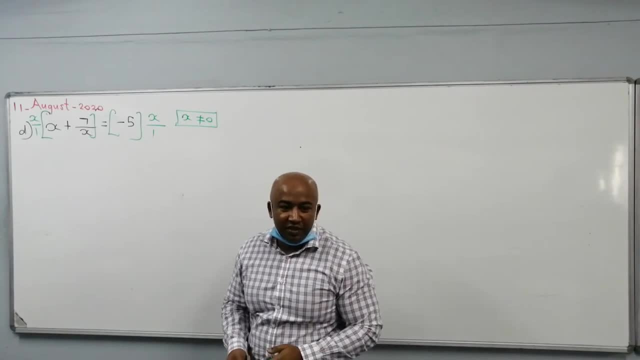 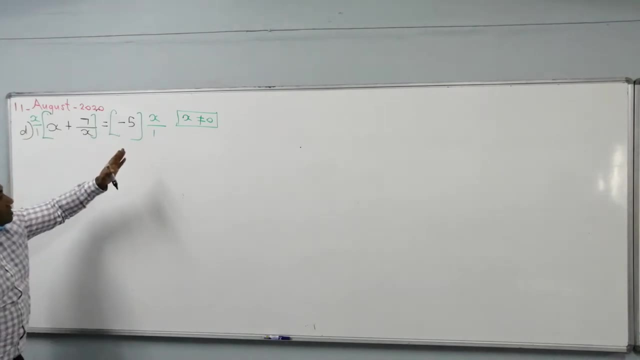 x cannot equal to 0, because you can't divide by 0. it's undefined. so now let's multiply on both sides. so why are we multiplying by x? because I want x in the bottom and x on the top, so cancel. that's why I am multiplying by x. 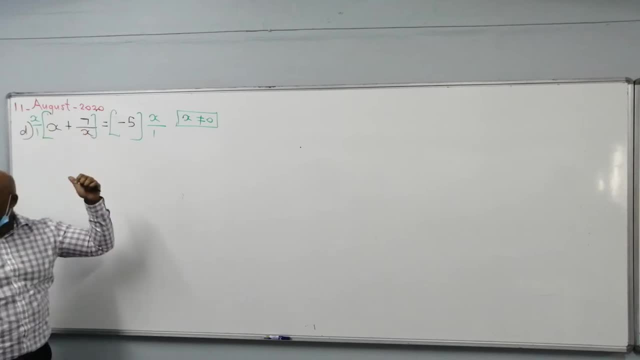 so whatever I do to one term, I need to do to every single term on both sides. so x times x will give me x squared x times 7 over x. this is 1 over x where x cancels now. so you get just plus 7 on the right hand side. minus 5 times x is 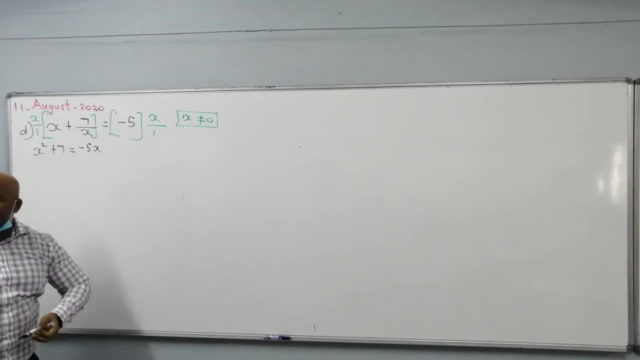 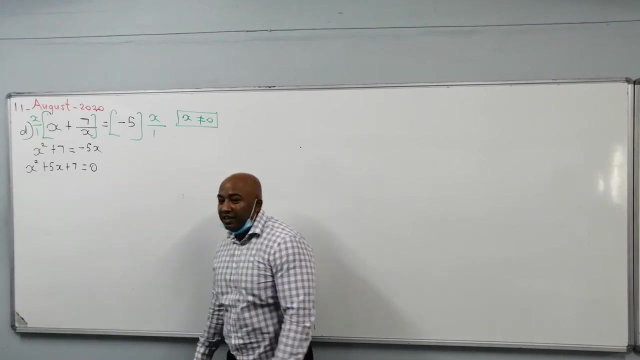 minus 5x and now make the whole equation equal to 0. so x squared plus 5x plus 7 is equal to 0. now you can see the factors of 7. 7 is a prime number. it only has the factors 7 and 1. 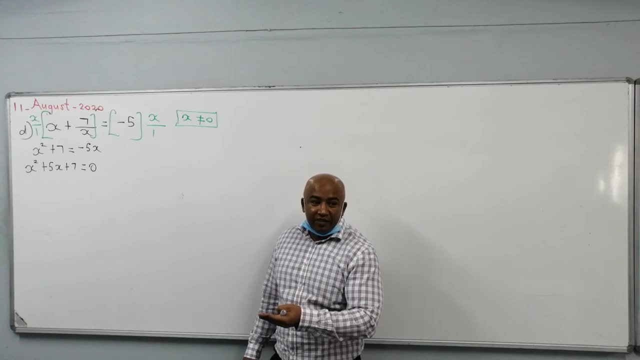 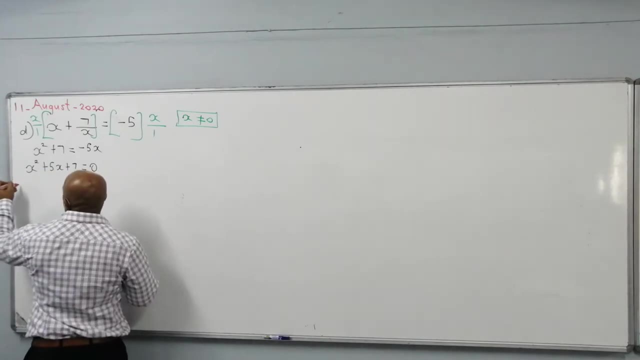 7 times 1 is 7, so we are not going to get 5. this cannot be factored, so we use the quadratic formula. the quadratic formula x is equal to minus b, plus or minus the square root of b squared minus 4ac all divided by 2a.